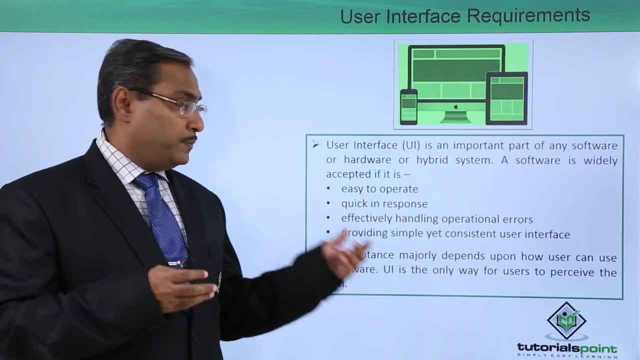 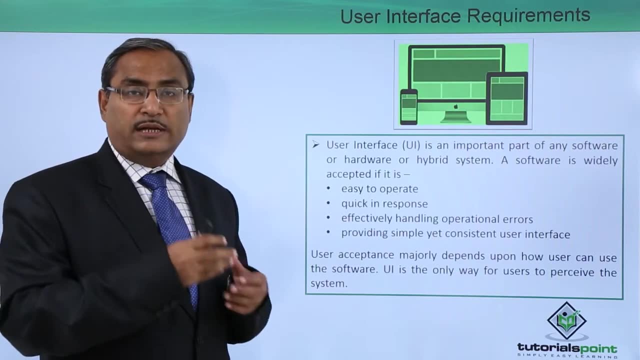 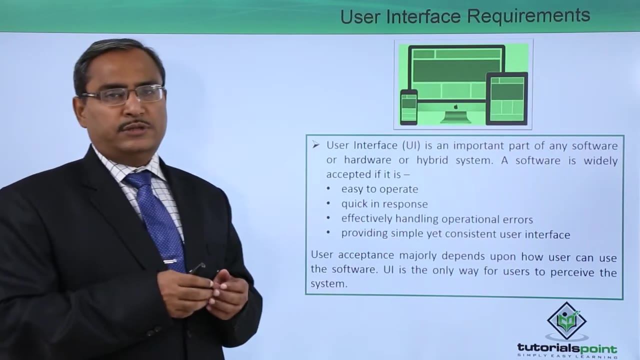 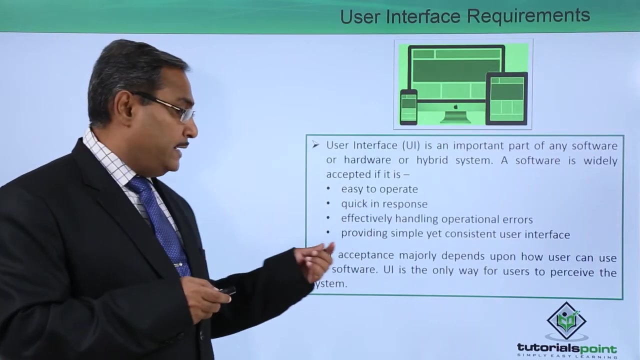 different errors will be generated, Then obviously the software must have the capability to handle that situation effectively and that may also give some guidance to the user so that user will not make such mistakes once again next time, And providing simple yet consistent user interface. User acceptance majorly depends upon how user can use the software, User interface in short. 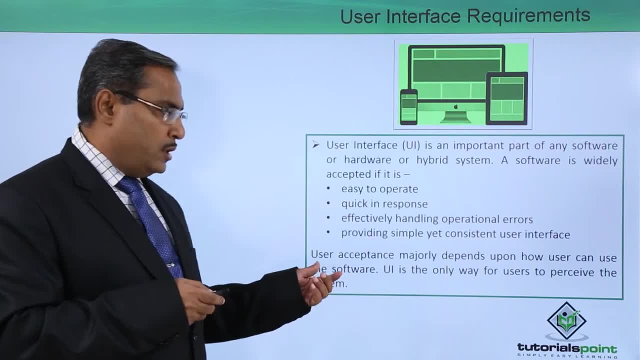 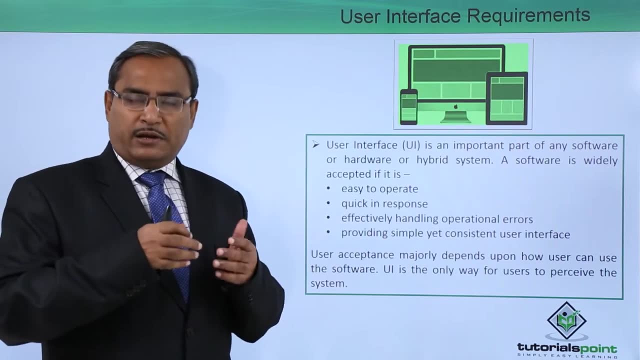 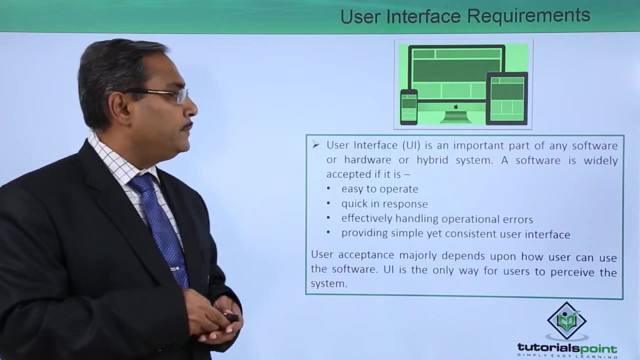 it is. UI is only way for users to perceive the system. So whenever user is interacting with the system, he or she can interact only through this UI. So this UI allows the user should be very much easy to operate and should be comprehensible. So a well defined or well. 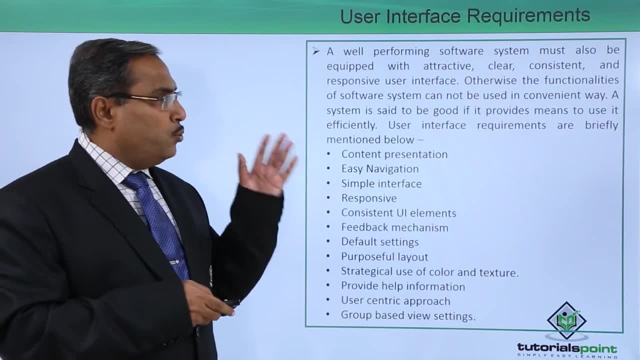 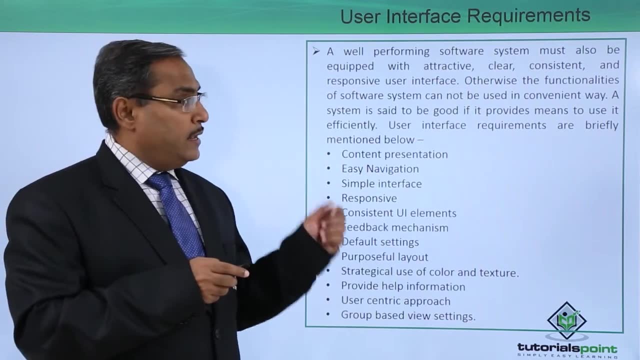 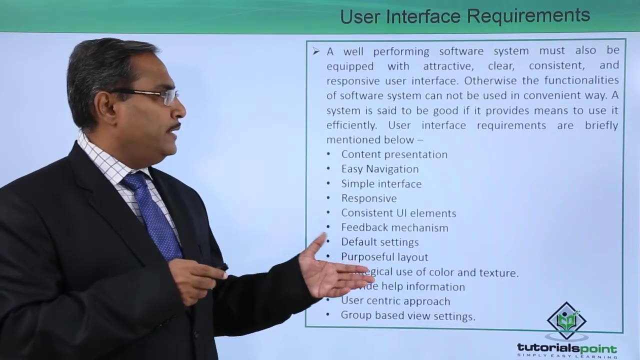 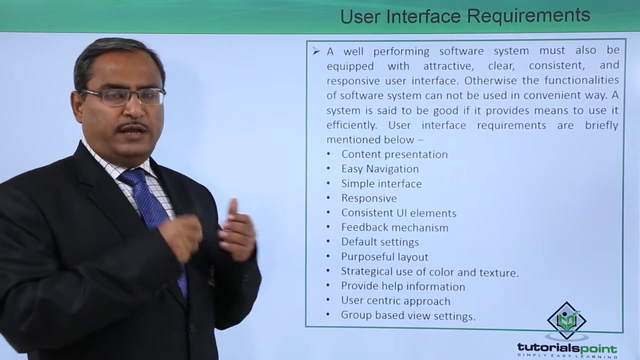 performing software system must also be equipped with the attractive, clear, consistent and responsive user interface. Otherwise, the functionalities of a software system cannot be used in a convenient way. A system is said to be good if it provides means to use it efficiently. So if user can use the system efficiently, then you can say that, yes, the 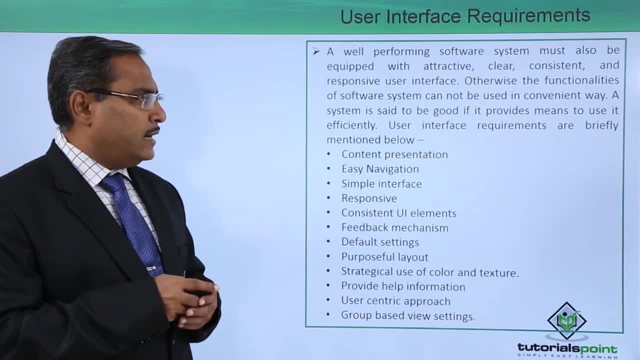 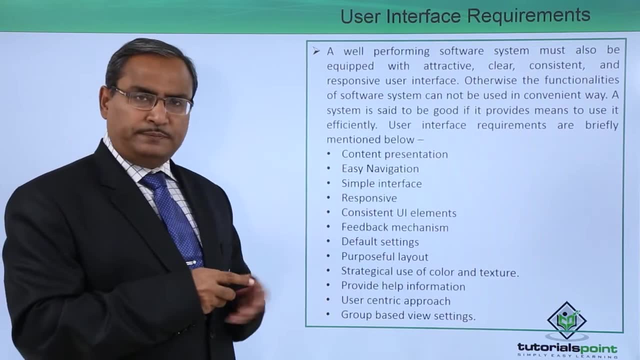 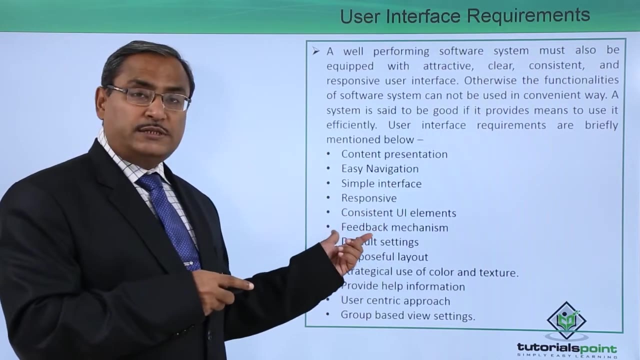 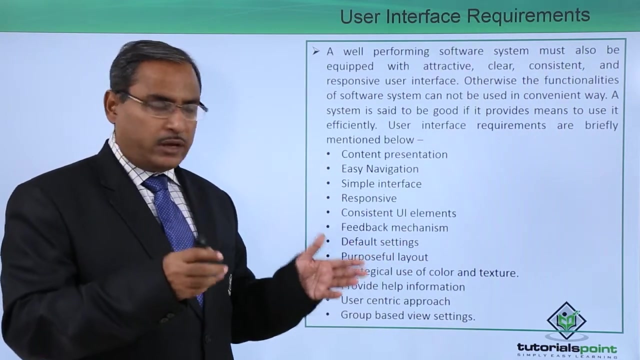 system is good for the user. User interface requirements are briefly mentioned below. So what are the user interface requirements? So: content presentation, easy navigation, simple interface, responsive, consistent UI elements. feedback mechanism: default settings should be in accordance to the user's requirement. purposeful layout: the layout should be also purposeful. 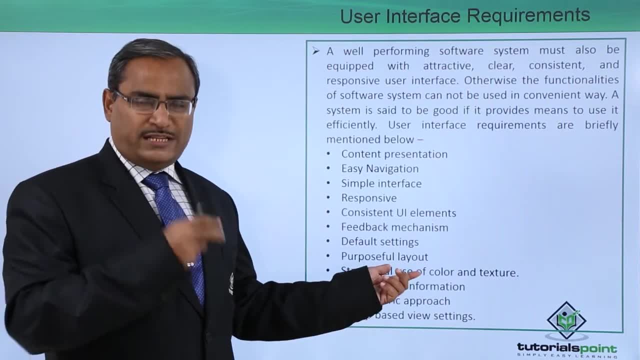 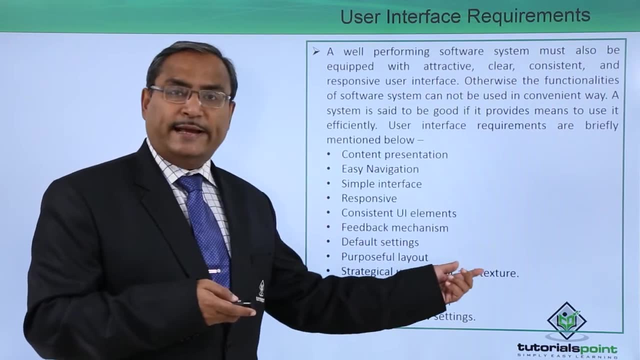 there are different layouts are possible. So which layout will be applicable for which user interface? that should be intelligently selected. So, strategical use of colors and textures. do not think that if you give on, if you make the user interface too much colorful, 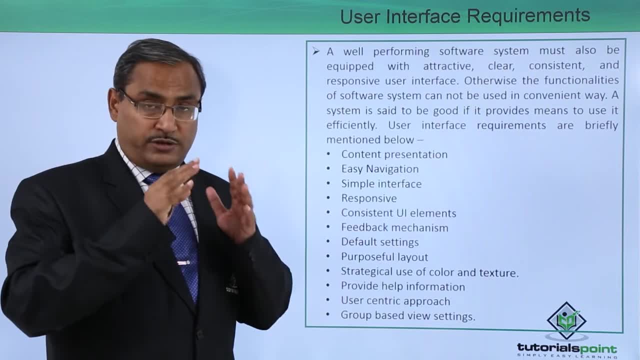 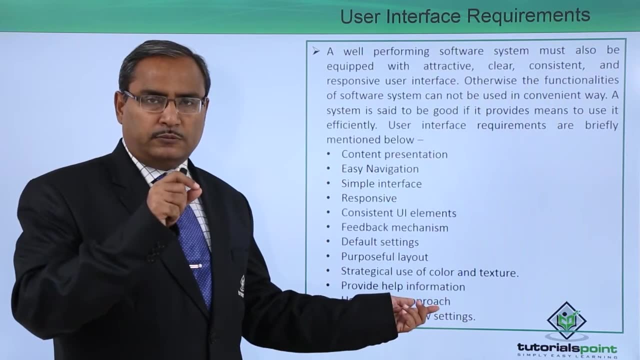 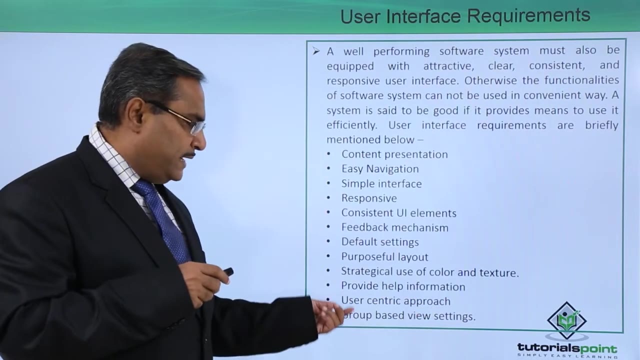 then it will be attractive. So simple, very plain, gentle interface will be an attractive one also. So provide help, information, so the help, what will be obtained from the software must be very much precise and should be purposeful and user centric approach and group best view.